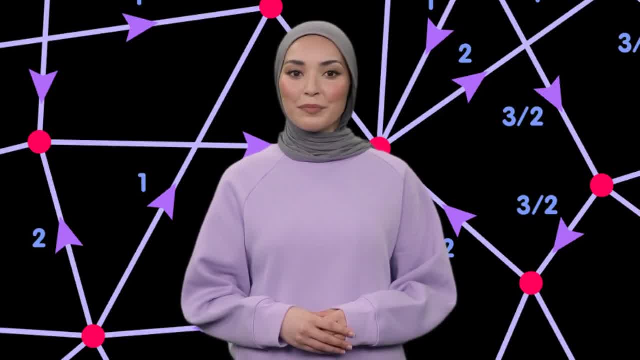 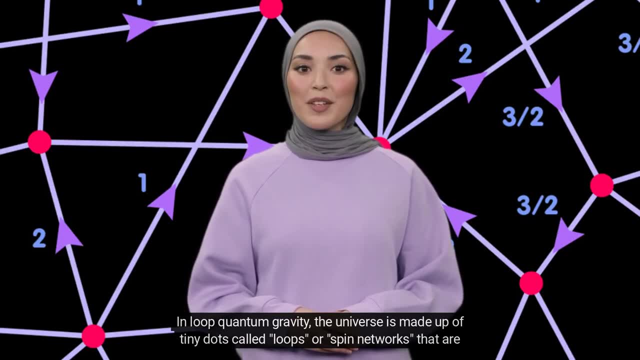 This is a bit like how loop quantum gravity works. In loop quantum gravity, the universe is made up of tiny dots called loops or spin networks that are so small that they can't be seen even with the most powerful microscope. These loops are constantly moving and interacting with. 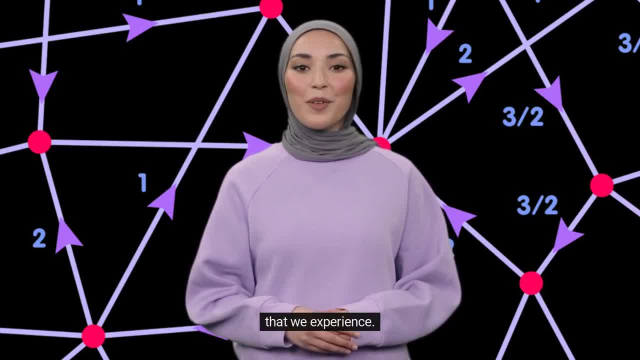 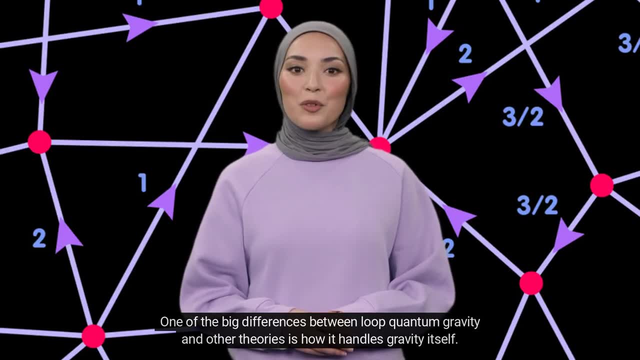 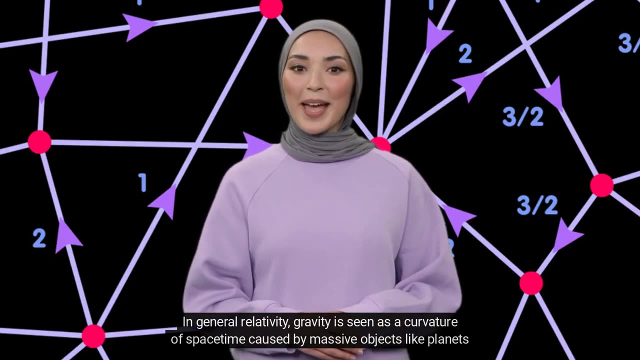 each other, creating the fabric of spacetime that we experience. One of the big differences between loop quantum gravity and other theories is how it handles gravity itself. In general relativity gravity is seen as a curvature of spacetime caused by massive objects like planets or stars, But in loop quantum gravity, gravity is seen as a force. 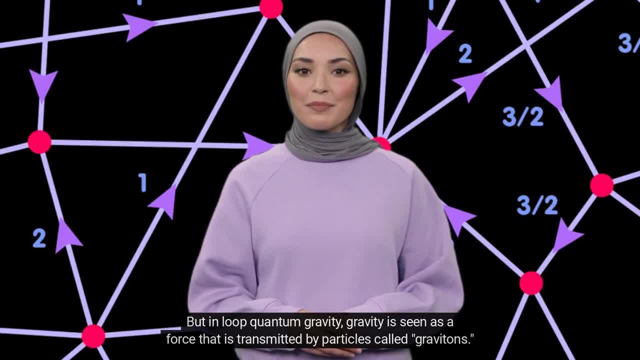 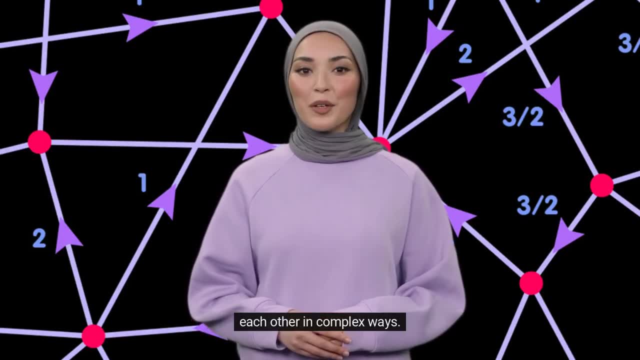 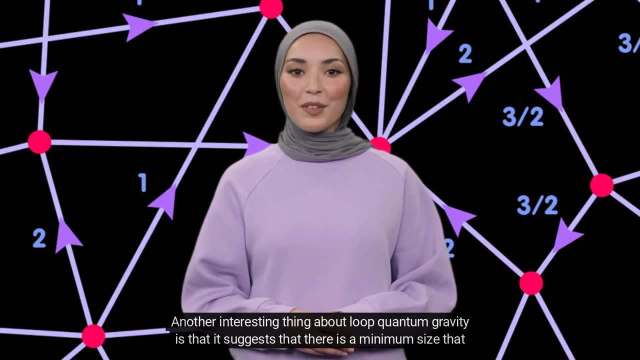 that is transmitted by particles called gravitons. These gravitons are constantly being exchanged between the loops, causing them to move and interact with each other in complex ways. Another interesting thing about loop quantum gravity is that it suggests that there is a minimum 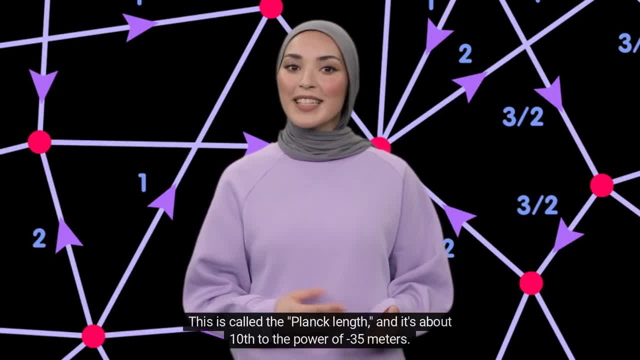 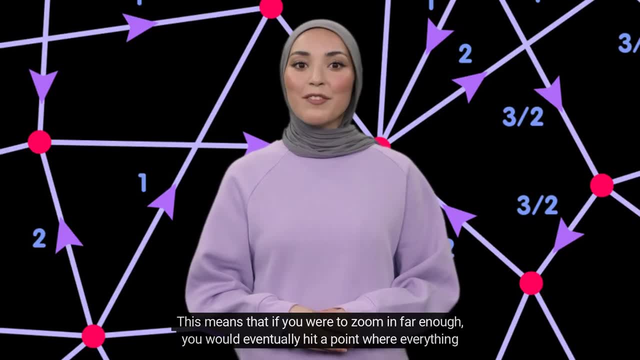 size that anything in the universe can be. This is called the Planck length, and it's about 10th to the power of minus 35 meters. This means that if you were to zoom in far enough, you would eventually hit a point where everything is made up of these tiny loops. 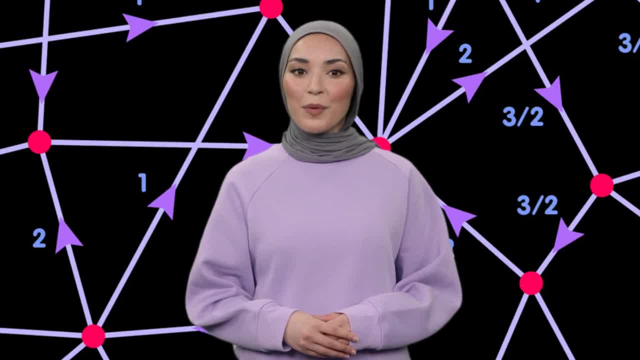 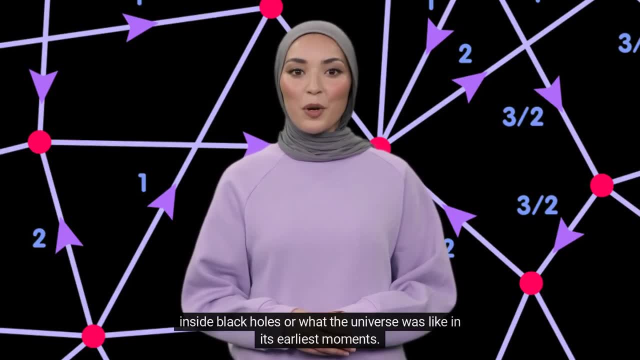 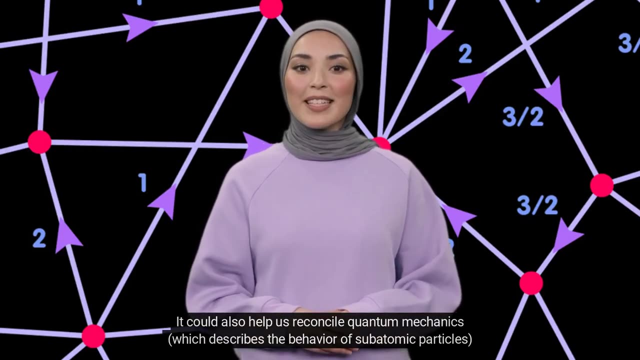 So why is loop quantum gravity important? Well, for one thing, it could help us understand some of the mysteries of the universe, like what happens inside black holes or what the universe was like in its earliest moments. It could also help us reconcile quantum mechanics. 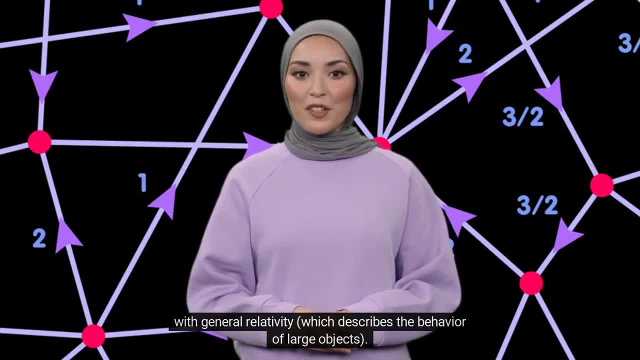 which describes the behavior of subatomic particles, with general relativity, which describes the behavior of large objects. One of the key challenges in combining these two theories is that quantum mechanics treats spacetime as a fixed background, while general relativity treats it as a dynamic and fluctuating entity. Loop quantum gravity resolves this tension by 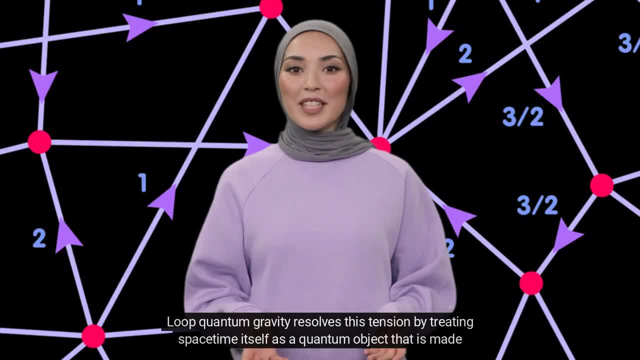 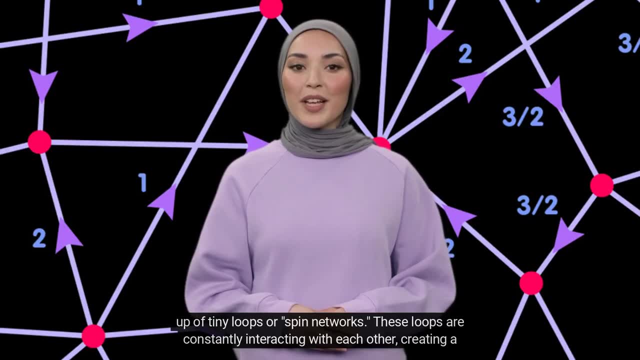 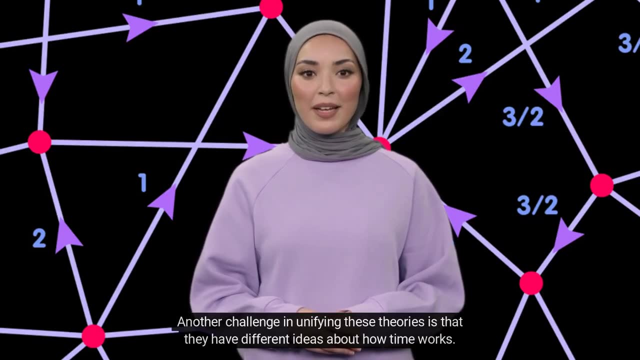 treating spacetime itself as a quantum object that is made up of tiny loops or spin networks. These loops are constantly interacting with each other, creating a web-like structure that represents the fabric of spacetime. Another challenge in unifying these theories is that they have different ideas about how time works. Quantum mechanics assumes that time is.